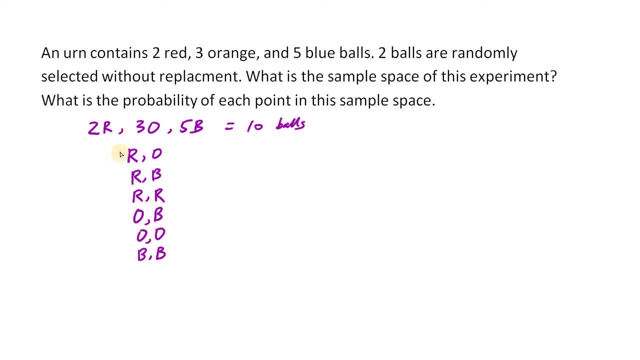 The sample space. So these six different outcomes represent the six points in the sample space, Six points of this sample space. So for the first one, the probability equals to two over ten times three over nine Times two x 3.. Times two: 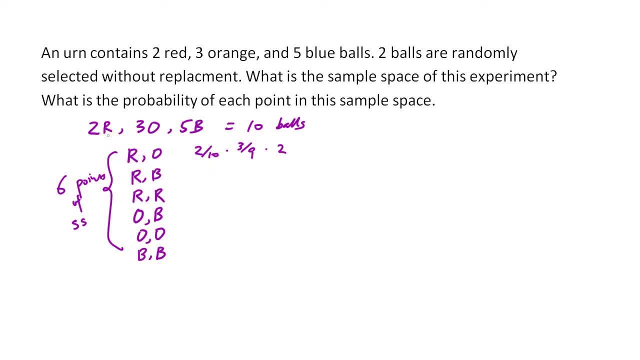 Why is that? First of all, we are going to choose a red ball out of the ten balls, So that we know will be two out of ten. After the first ball is chosen, we are going to select an orange ball from the remaining ball. 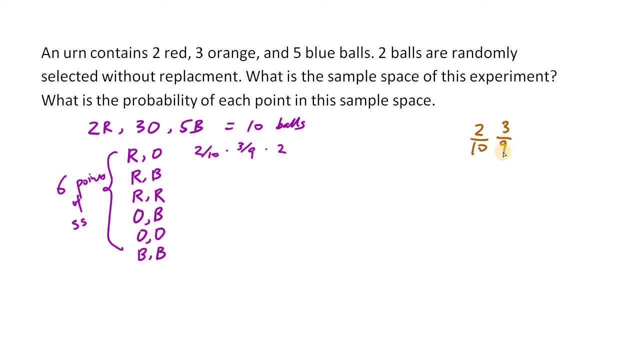 which is three of the nine balls left. Well, if the order does matter, then this will be the probability of getting a red ball and then an orange ball. However, since order doesn't matter, we also need to add the case where we get an orange ball first. 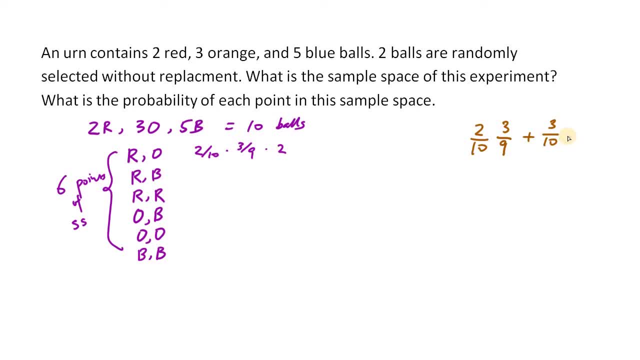 so, which would be three over 10, and then a red ball, second, which is two over nine. That's the answer for the first probability. So, similarly, for red and then blue, it will be two, choosing two from 10 balls and then choosing five from nine balls. 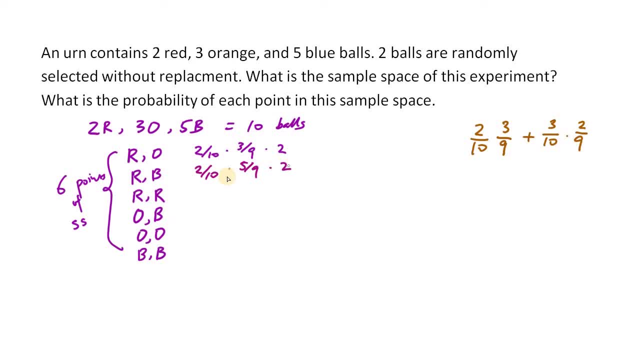 And then, since they are different balls, so there are two ways of getting this outcome, which is similar as the previous case, But to get two red balls, it will be two out of 10 times one over nine In this case, even if we swap the first ball. 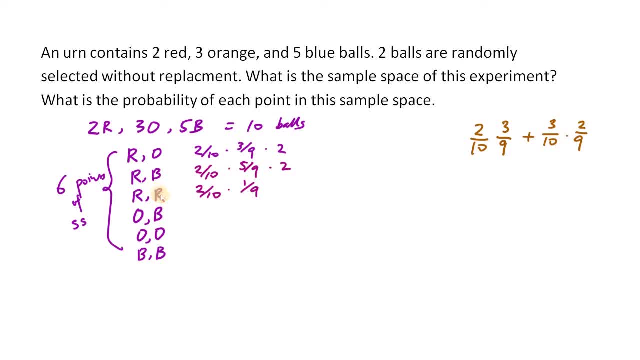 and the second ball. it's still considered the same outcome, So we don't actually multiply it by two. For the next case we're gonna get an orange and a blue. So three over 10 times five over nine. Orange well times two.